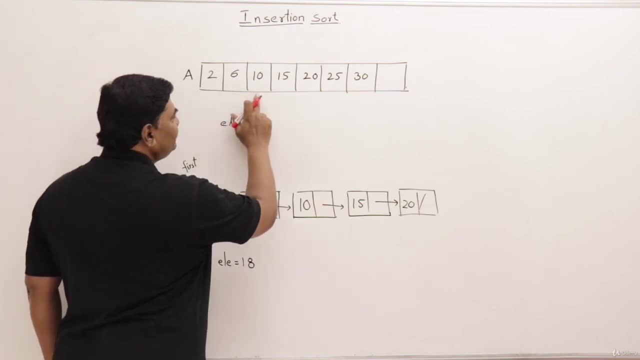 should come. So after 2,, after 6,, after 10,, yeah, before 15.. It should come here, 12 should come here. Then insert 12 here. For inserting 12 here, what I have to do, I have to shift all these. 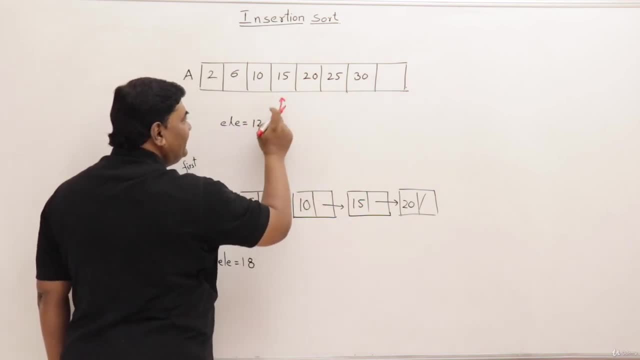 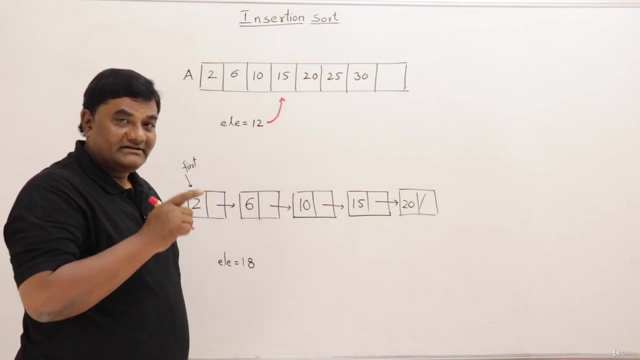 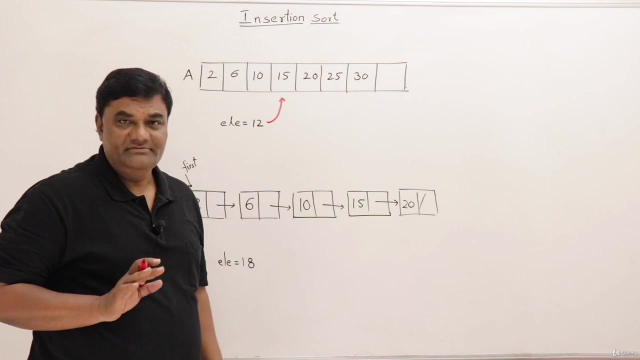 elements on the right hand side. Make a free space here, then insert 12.. So if you observe what I have done, I first found out where 12 should come, Then I said I will be shifting the elements. So the important thing is you don't have to find out where it should come Directly, you can start. 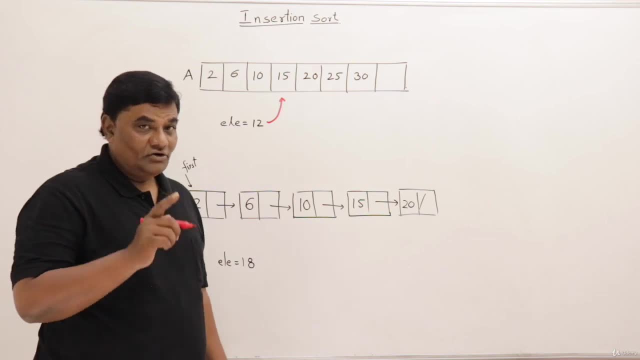 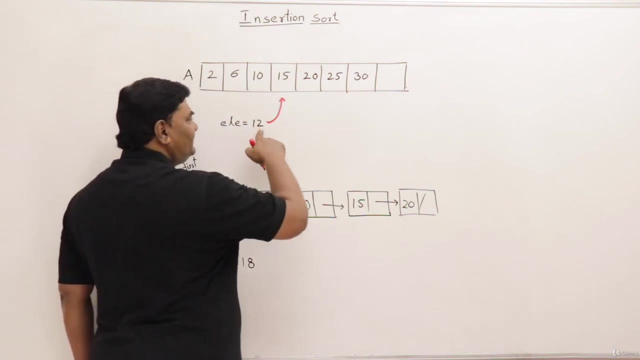 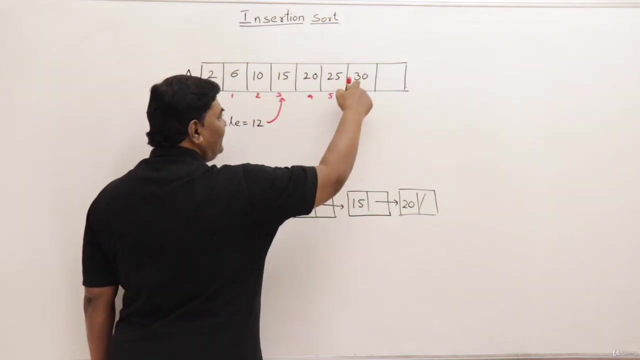 shifting the elements. You don't have to find its position Now. I will show you exact procedure, how this insertion should work. Let us start. I want to insert 12.. The last element is at this index. I don't have indices. Okay, I will write down indices Now. last element is at index 6.. 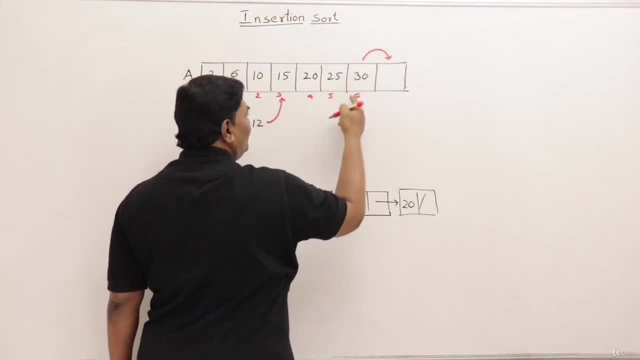 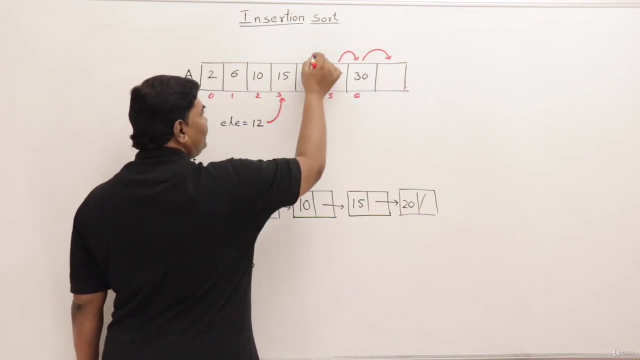 So is it greater than 12?? Yes, Shift it. Move to the next element: 25 is greater than 12.. Shift it. And next element, 20 is greater than 12.. Shift it. Next element: 15 is greater than 12.. Shift it, Then. 10 is not greater than 12.. So I am here now, right now. Okay, I have. 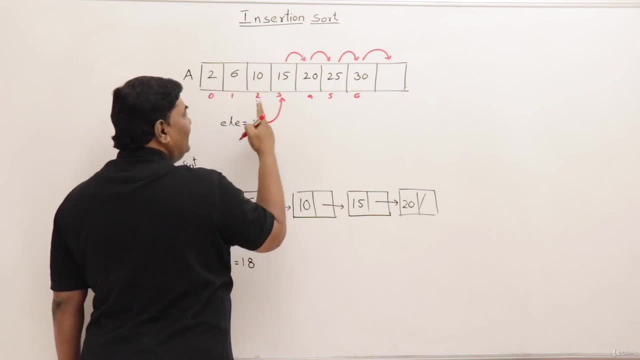 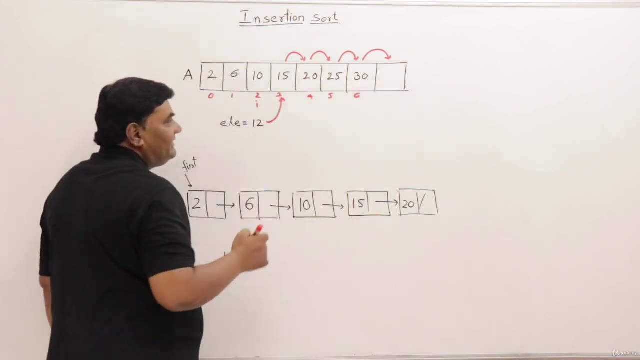 moved all the elements. Now, right now, here, 10 is not greater than 12.. So this place is free. So this place store the element 12.. So all these elements will be shifted and 12 will be inserted here, So I don't have to search and find out its position from the last. 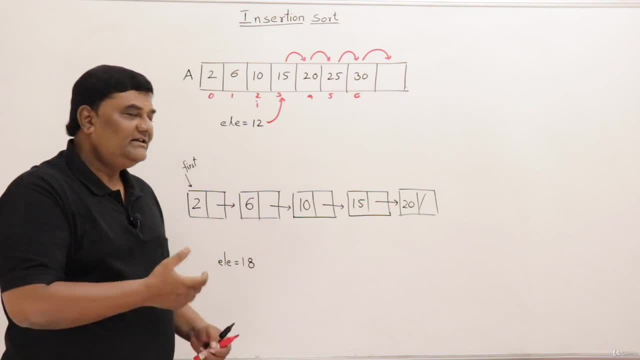 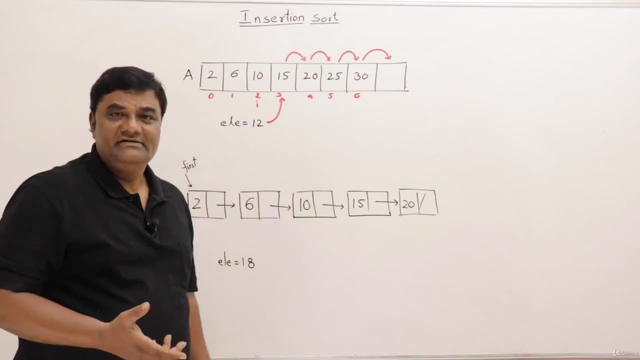 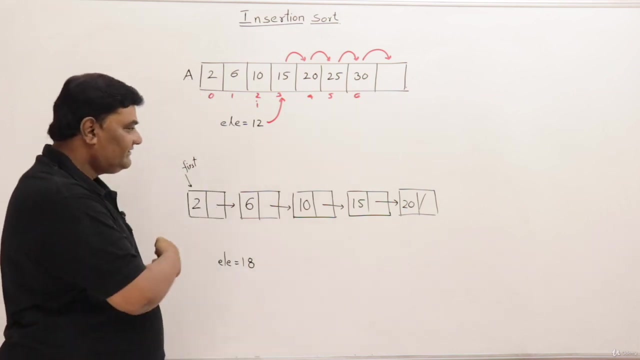 I am shifting larger elements. Then wherever you get any elements smaller than the element that you are inserting, insert the element there. So all the larger elements are shifted on the right hand side. That's all. This is insertion. Then let us also see insertion in a linked list. So I 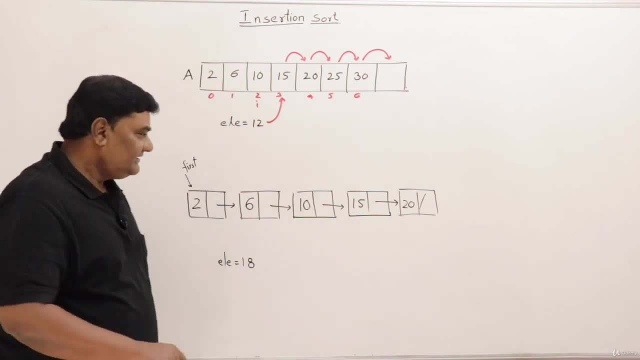 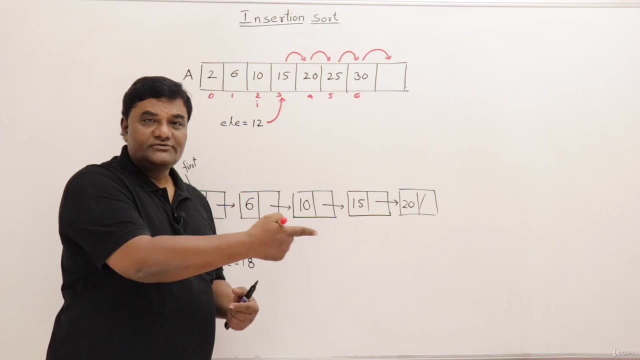 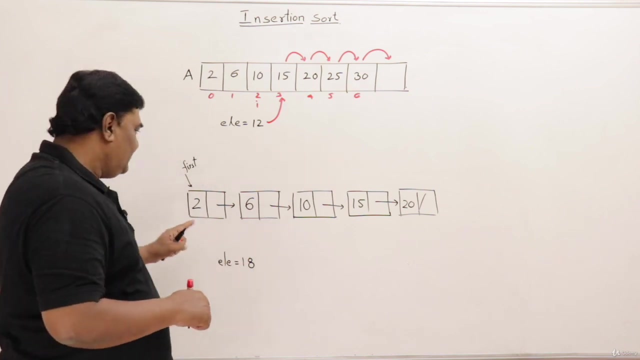 have taken a linear singly linked list and this is a list of sorted elements and I want to insert 18.. In a linked list we don't have to shift the elements. Shifting is not required. Then we have to find out where this 18 should come Like in this linked 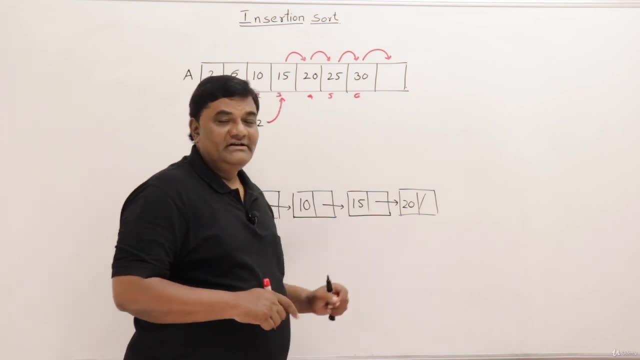 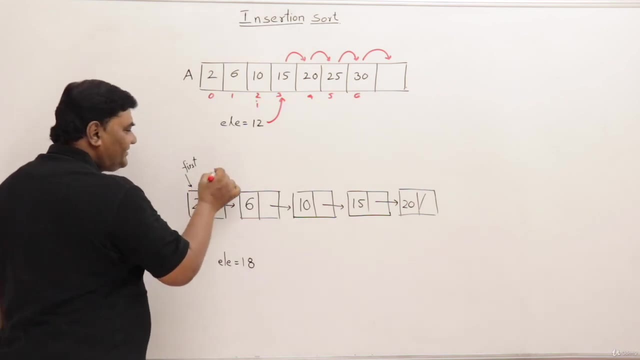 list 18 should come after 15 or before 20.. So I should find out its position and insert it. That's all. So for finding its position I will take a pointer to traverse a linked list. Then also I will take one tail pointer. Now I am showing you the procedure, how to insert it. Check P's data. 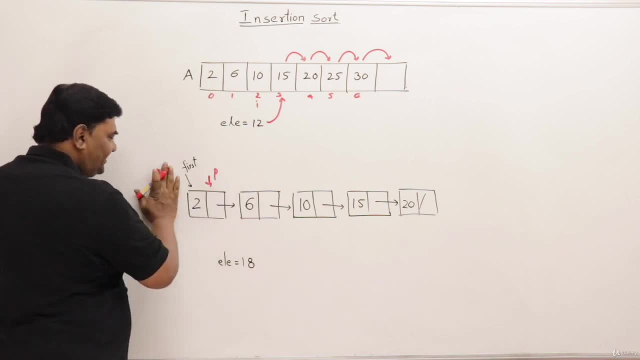 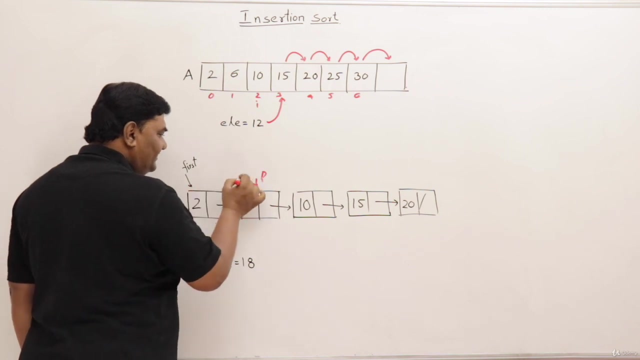 That is smaller than this one. So move P to next, But before that bring Q upon P and then move P. This is smaller than 18.. So again move P, But first bring Q upon P, then move P. Now P's data is smaller than 18.. Again move P and Q. So first Q, then 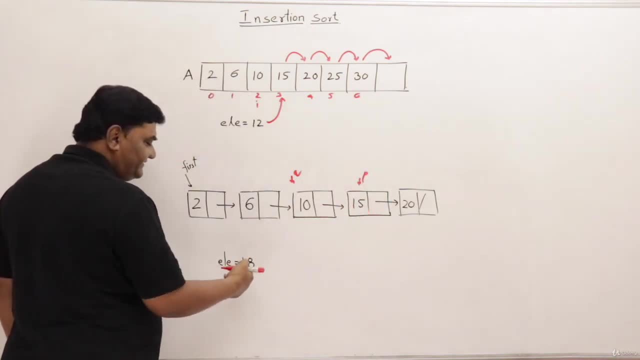 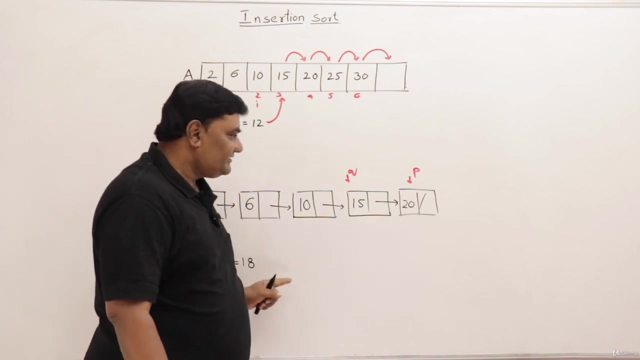 move P. This is still smaller. 15 is smaller than 18.. So move Q upon P and move P to next. Now, 20 is greater than 18.. So we have found the first element, which is greater than the key element that we are inserting. So we found its position. So it should be after Q. So for that, 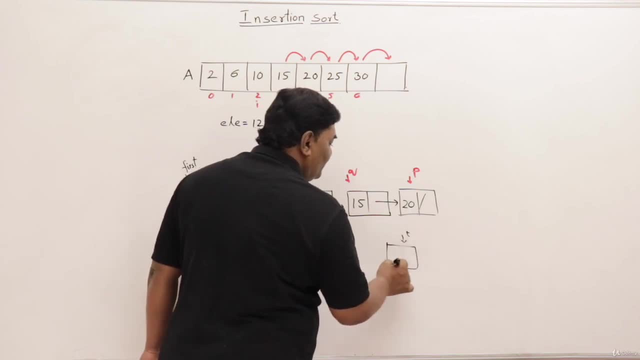 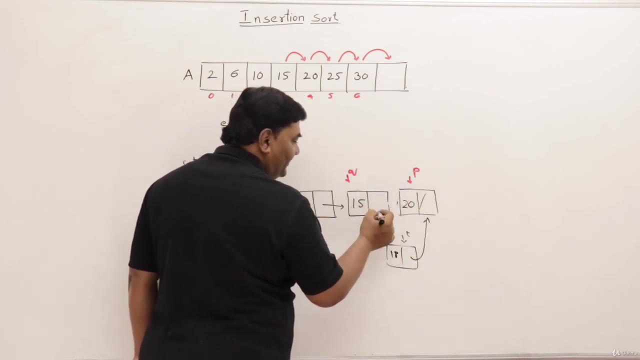 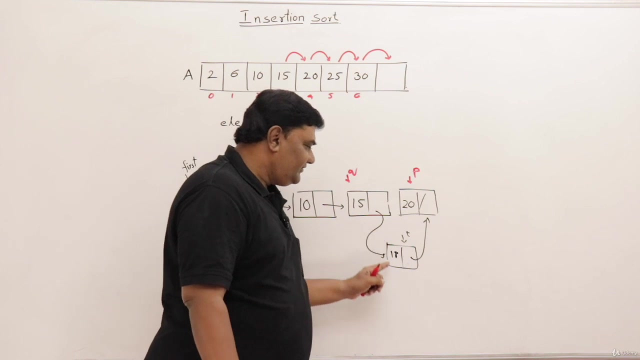 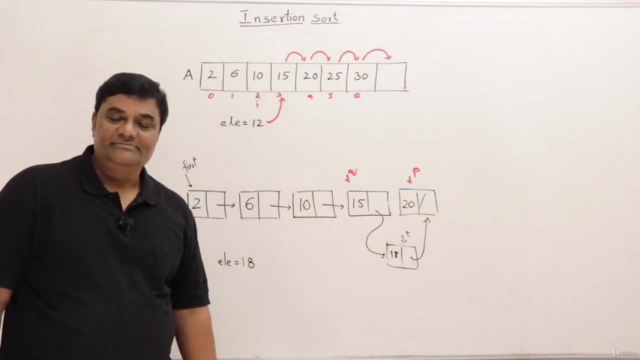 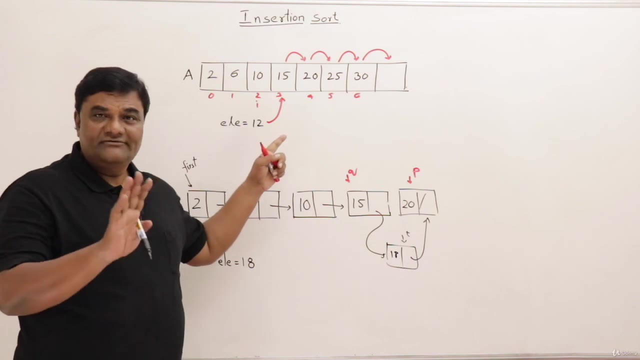 15 to 18,, 18 to 20.. So 18 is inserted in a sorted position. So in a linked list we have to find out its position and then insert, Whereas in an array we don't have to find the position, Simply shift. 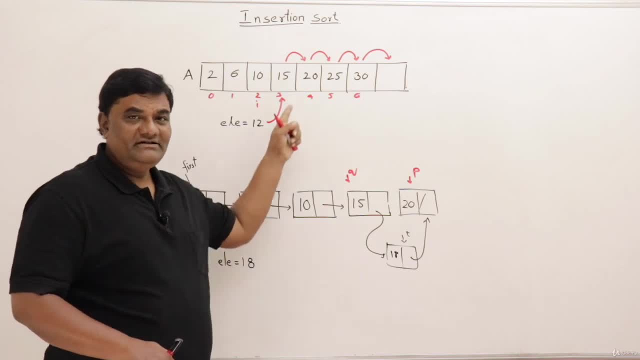 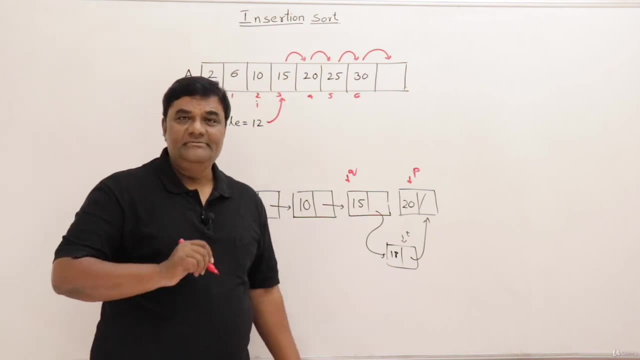 the elements and once you get a smaller element then insert, And once you have finished shifting all larger elements then insert at a free space. So what is the time taken for insertion in an array? Shifting of elements, How many elements? Some elements. 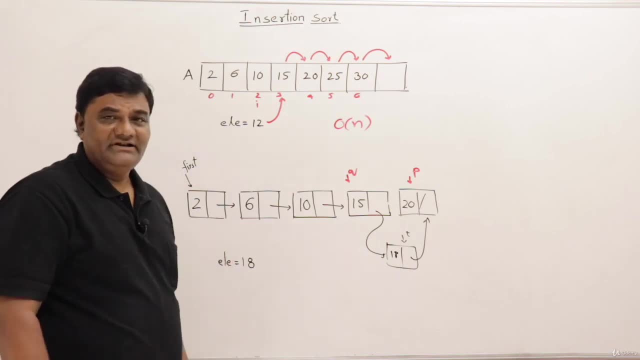 Some elements are shifted, So n depends on the number of elements. Maybe zero elements are shifted, Maybe all elements are shifted, So it may be minimum constant, maximum n, Minimum constant and maximum n. Then here find out the position using P and Q. So traversing takes time. Insertion.